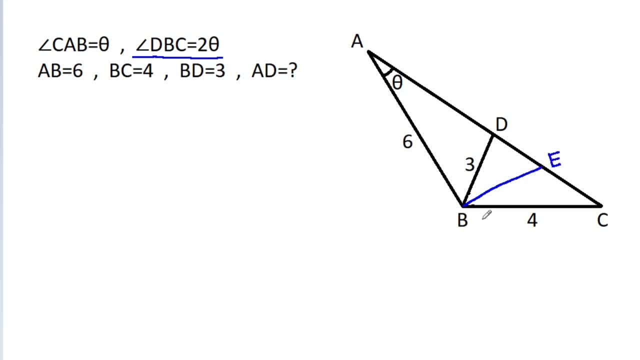 suppose this is point. is E such that these two angles are theta, then in any triangle A, B, C, if AD bisect this angle, then A, B by AC it is equal to BD by CD, And also AD squared it is equal to AB times AC, minus BD times CD. 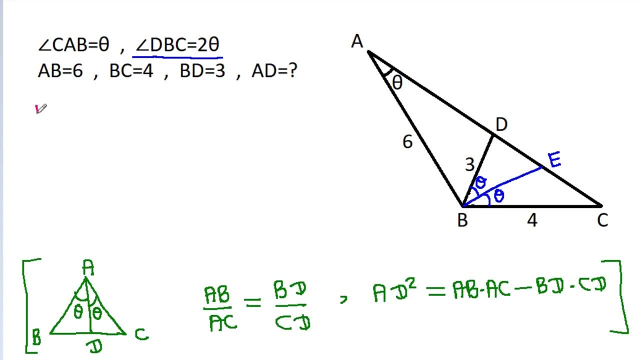 So here in triangle BDC, DE by CE it will be equal to BD by BC, and BD is 3 by BC is 4.. That means if DE is 3Y, then CE it will be equal to 4Y. 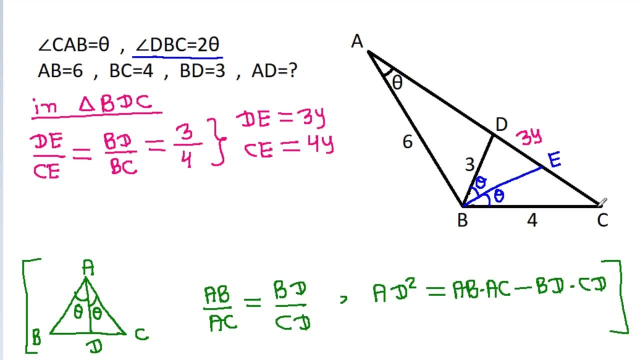 If DE is 3Y, then CE it will be 4Y And also BES squared it will be equal to BD. That means this is 2.. So next in triangle it will be equal with DE by CE. 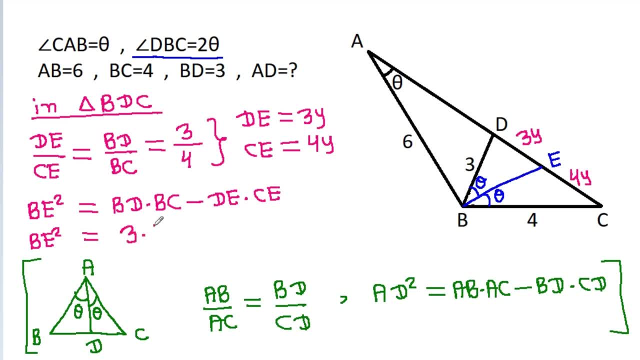 That means DE by CE times BC, minus DE times CE. So BE squared. it is equal to: BD is 3, times BC is 4.. Minus DE is 3Y times CE is 4Y And it is 2N. 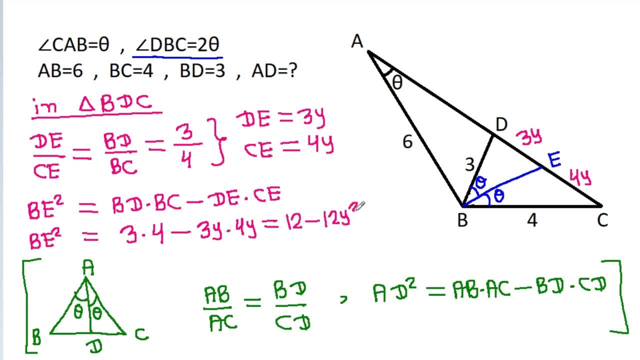 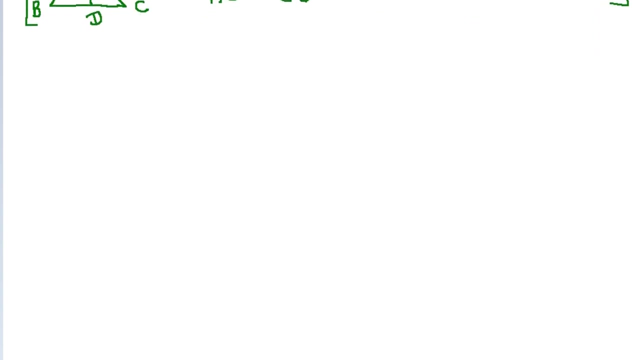 So I considered this teuco 2n minus 12 y square, So b? e it will be a square root of 12 minus 12 y square. And now in triangle ABC and triangle BEC, angle BAC, it is equal to angle EBC, that is triangle. 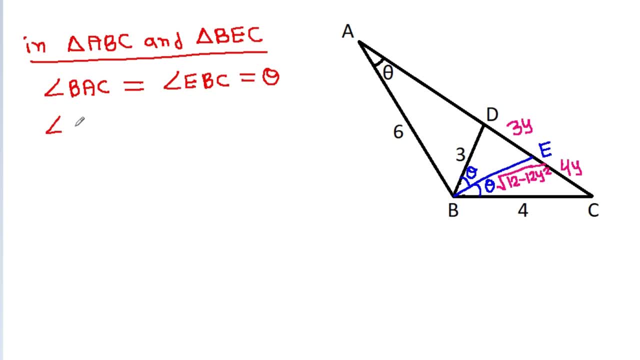 theta And angle ACB it is equal to angle BCE. it is common. So by angle angle similarity, triangle ABC it will be similar to triangle BEC, hence AB by BE it will be equal to BC. by EC and it will be equal to AC by BC and AB is 6 by BE is a square. 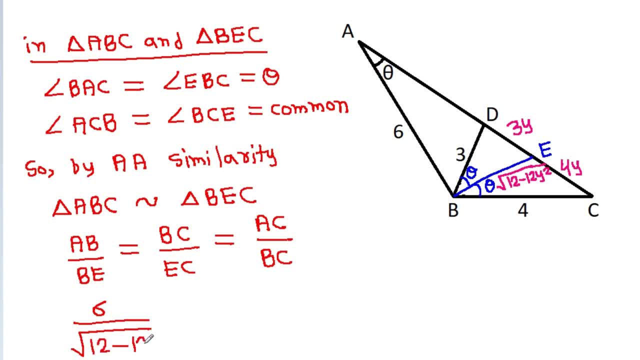 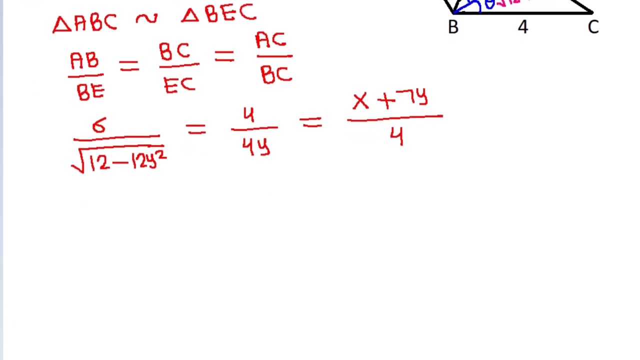 root of 12 minus 12 Y square it is equal to: BC is 4,. by EC is 4Y, it is equal to AC. suppose AD is X, then AC, it will be X plus 3Y plus 4Y. that will be X plus 7Y by and BC is 4,. and from this equation, if we 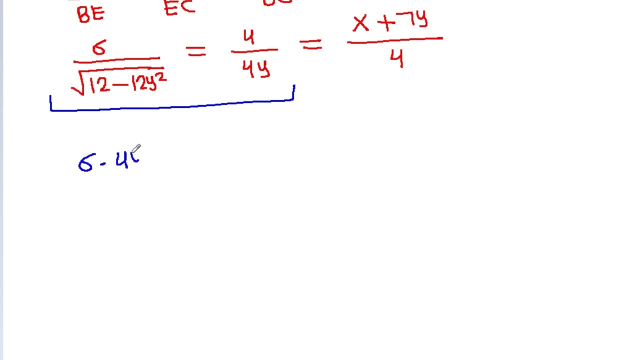 cross. multiply then 6 times 4Y, It will be equal to 4 times a square root of 12 minus 12Y square, and 4 will get cancelled. so 6Y it will be equal to a square root of 12 minus 12Y square. and if we square it, 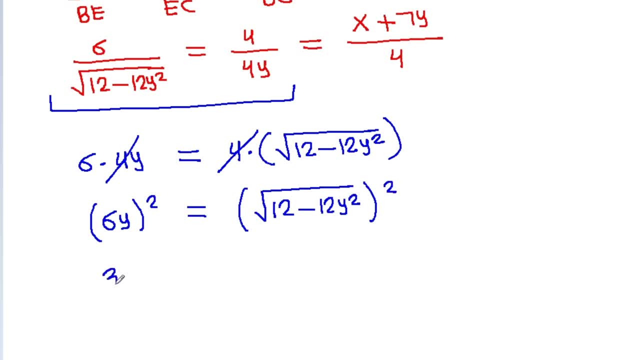 both side. then it is 36 y square is equal to, and here a square and a square root will get Slant. So it is 12-12 y square and 36 y square minus 12 y square, It will be equal to 12.. 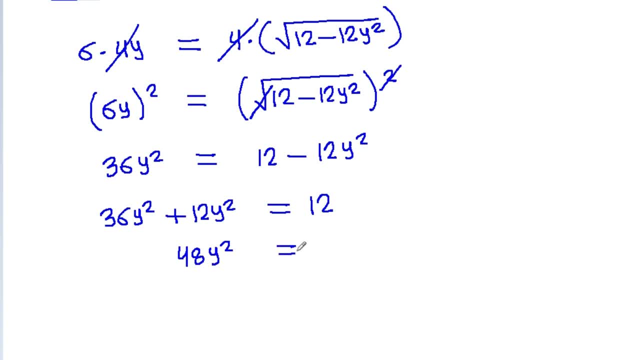 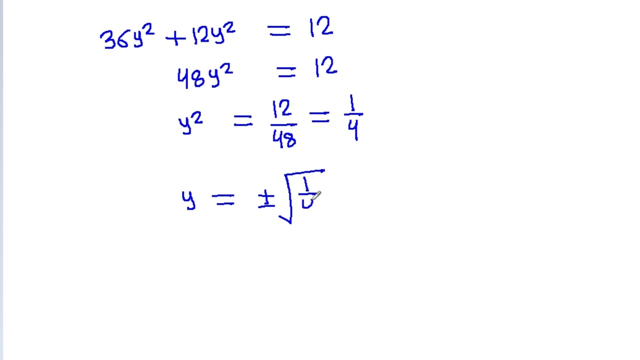 And it is 48. y square is equal to 12. so y square will be equal to R square plus 2env by 48. that is equal to 1 by 4.. So y will be equal to plus minus s square root of 1 by. 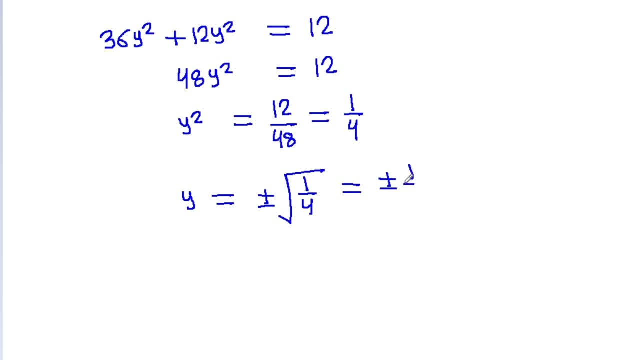 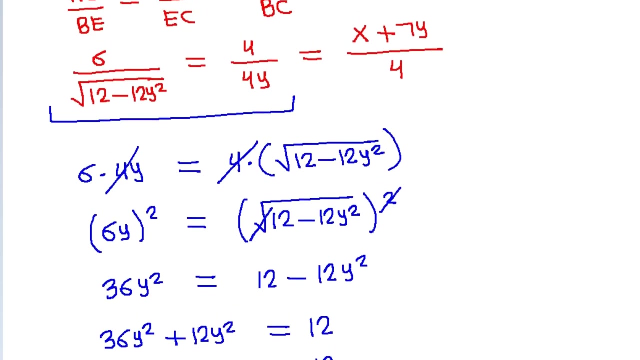 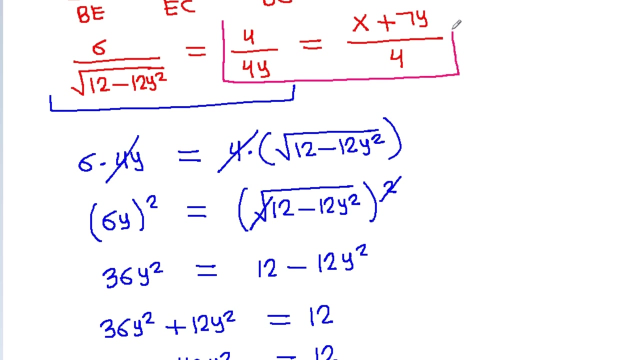 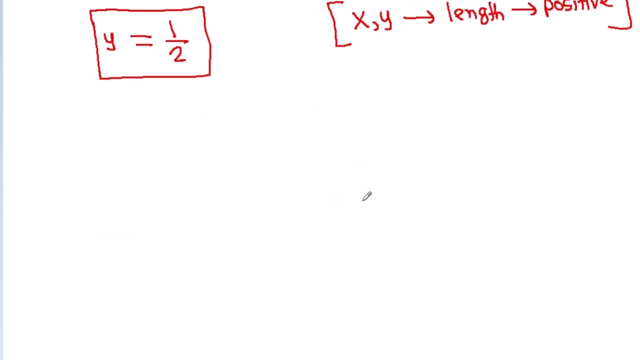 4, that is equal to minus minus 1 by 2.. And x and y, they are length. that should be positive. So we get y is equal to 1 by 2.. And we have 4 by 4: y is equal to x plus 7 y by 4.. We have 4 by 4: y is equal to x plus 7 y by 4..